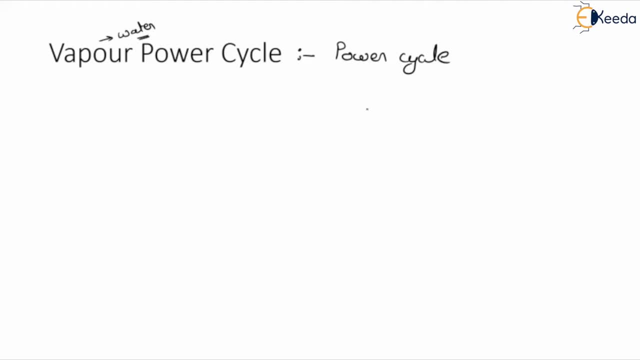 a cycle where the heat energy which comes from the burning of fuel, it will convert into work, where the working fluid is performing a complete process. So what is power cycle, Power cycle? here working fluid will perform the complete cycle and here we will get the heat energy by burning the. 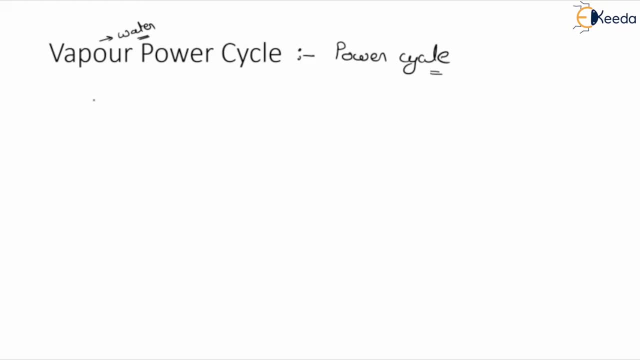 fuel and it will further convert into work. So here what is happening: We are getting heat from particular source and we are converting this heat into work with the help of working fuel or working fluid. So this is the main process of power cycle: Heat is converting into work with the help of 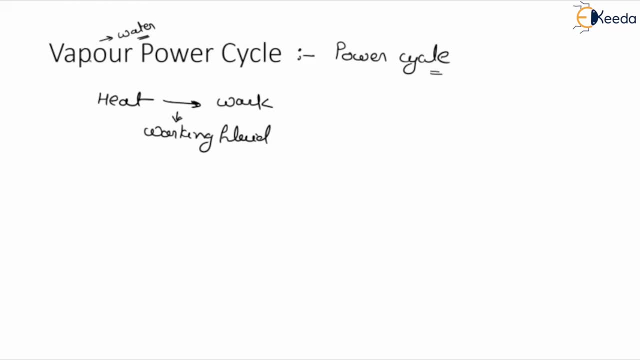 working fluid. So that is called power cycle. Now why it is called vapor power cycle? Because this working fluid we are considering as water, vapor or water. that is why it is called vapor power cycle. Suppose if we are using any kind of gas as a working fluid, so it will become gas power cycle. 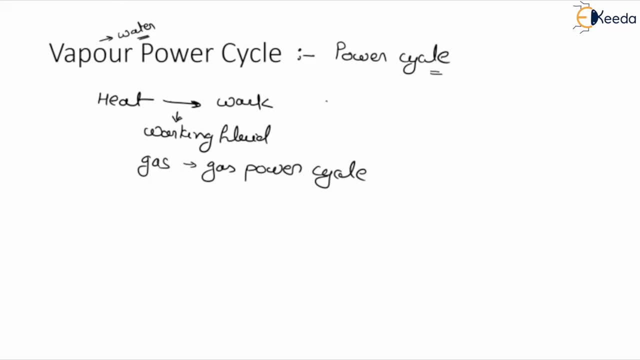 So by changing the type of working fluid we can change the type of power cycle. So here our main working fluid is water vapor, so that is why it is called vapor power cycle. Now, if we talk about vapor power cycle, So 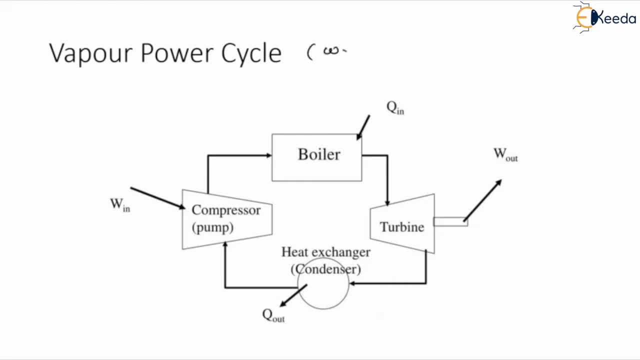 working fluid is here. What is the working fluid? The working fluid is always considered as water and water here. we cannot use water directly for the power generation. First we need to change the phase of water, So this water will further convert into steam or water vapor. 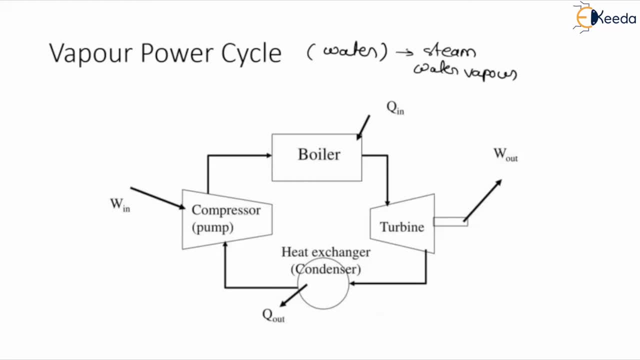 So we cannot directly use this water. So what is happening here? The water is changing the phase, So there are various phase changes we have to consider during the whole process. So here, water in the form of different phases we have to use to generate the power or to convert heat. 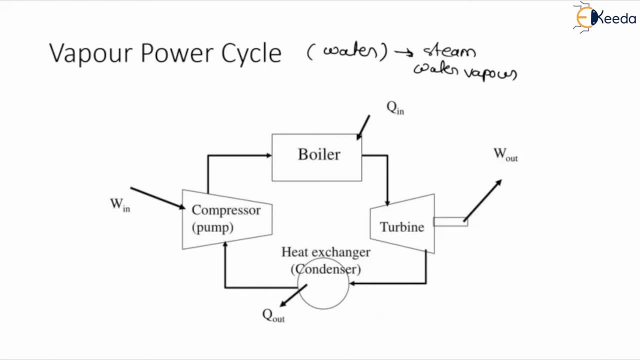 into the work. So this is the basic working of the vapor power cycle. Now here if we talk about the example. So example is mainly we can take as steam power plant. So steam power plant work on vapor power cycle. The working of the steam power plant we can define on the basis of: 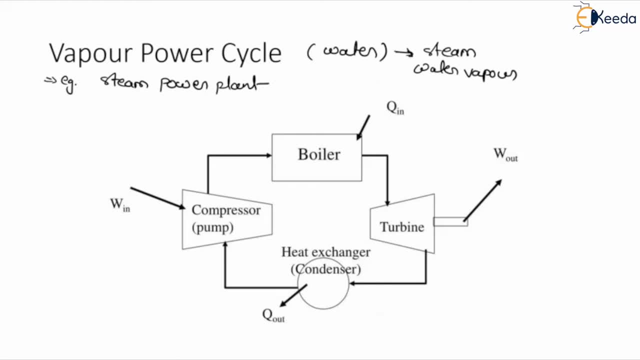 vapor power cycle. So here in this diagram you can see, this is the diagram. In this diagram we will define the simple working of steam power plant. So here you can see. there are number of parts mentioned here: Boiler turbine, heat exchanger or condenser and compressor. So let me write down. 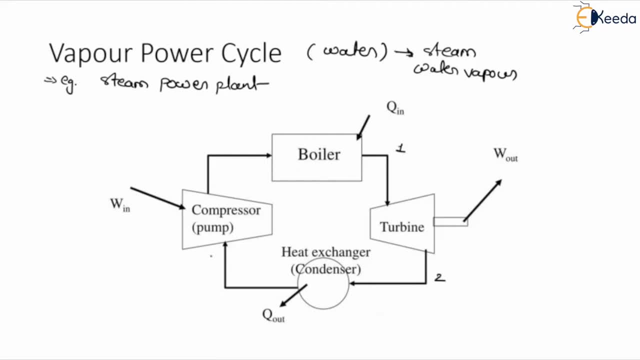 the processes. So suppose this is process number one, this is process number two, this is process number three and this is process number four. So here we will divide complete process into four processes or four states. So boiler turbine, condenser and compressor are the main parts or devices of the steam power plant. Now 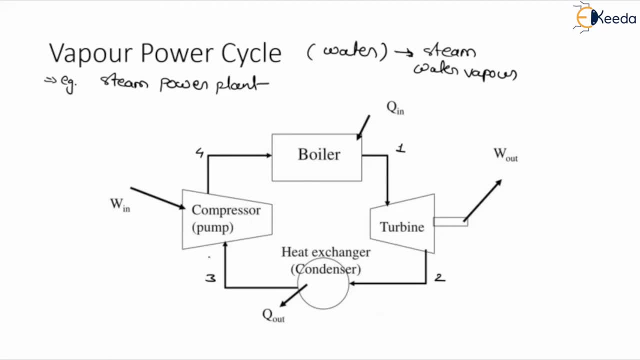 how the steam power plant work, or what is the basic theory behind the working of the steam power plant, or this is also called thermal power plant. So here I will tell you the complete working of the thermal power plant, how it actually work. So here you can see the first. 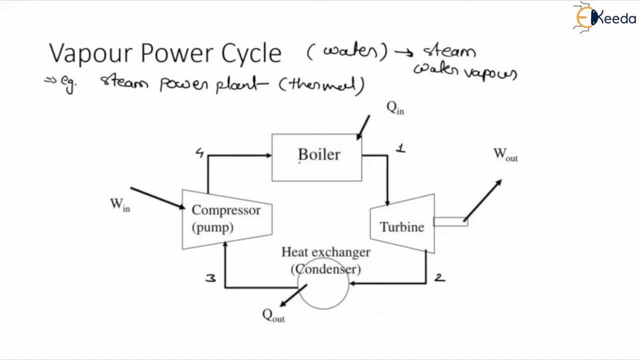 part that is called the boiler. So here you can see the first part that is called the boiler. So boiler means what? Where the fuel or the fluid boil? Basically, it is boiling the fluid. So what is the fluid we are using? We are using the fluid as water, So boiler will boil the water and from the boiler we will get high temperature and high pressure steam. Now how we are going to boil this water. So this water will boil with the help of some external 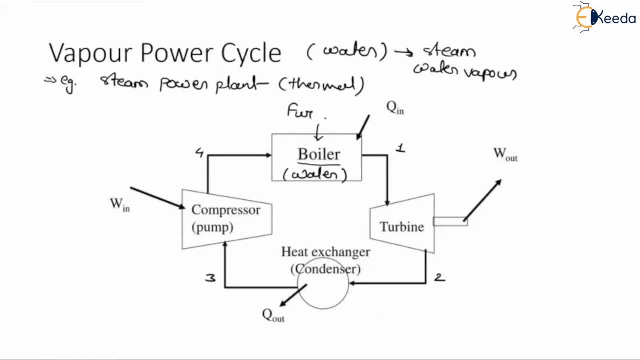 heat source. So this external heat source we can take as furnace. So from furnace we will get the heat. That heat will boil the water here and this water will convert into the steam or water vapor. And here what is happening? heat addition. So Q. 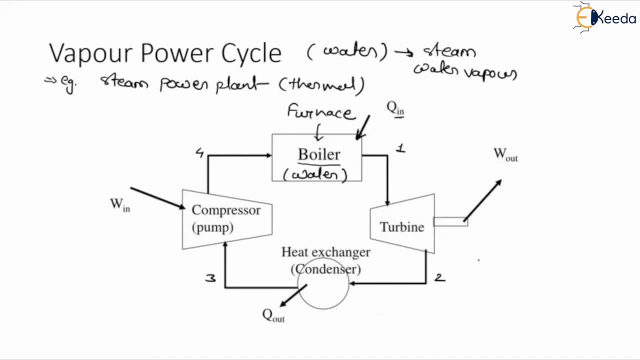 in This Q in is representing what it is representing: the heat addition. So this heat is generating the high pressure, high temperature steam, and this particular heat we are getting from external heat source that is called the furnace. So now, here in this process, when we will get the high pressure, high temperature steam from the boiler? 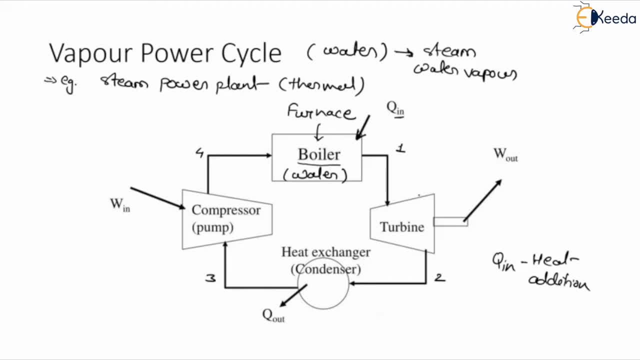 it will transfer to the turbine. So this high pressure, high temperature steam is it will transfer to the turbine for further process. So this process we are considering as process number one: transfer of high pressure, high temperature steam to the turbine. and this particular process is defined as process of heat addition. So this Q in we are considering as the process or the 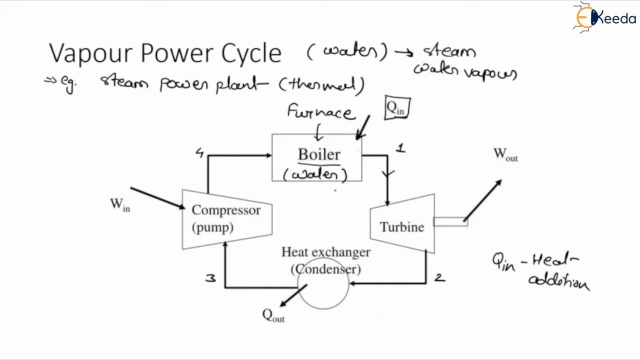 first process for this steam power plant. So this high pressure, high temperature steam from the boiler, it will transfer to the turbine and in this turbine the steam will expand, and how it will expand. So this turbine consists number of parts, So it consists one rotor or impeller and there are 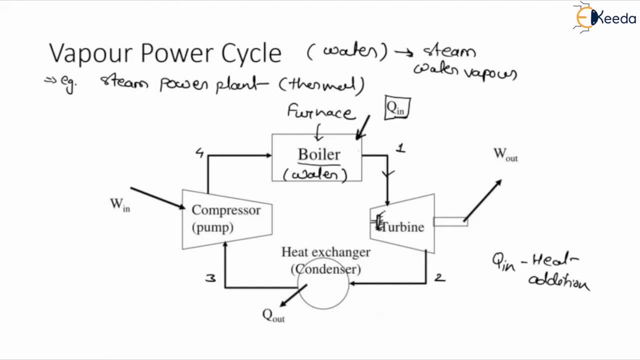 number of blades situated on this particular rotor or impeller. So what will happen? This high pressure, high temperature steam, with high pressure, it will hit the blades of the rotor. and what will happen? Because of the pressure of this steam, this rotor will rotate and this rotor 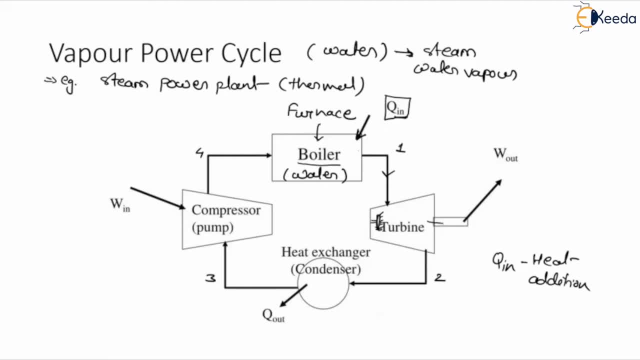 will rotate and it will further connect it to the shaft. So this shaft will transfer the power to the turbine. So this is the number of blades situated on this particular rotor or impeller. So this high pressure, high temperature steam will transfer the power to another device. This 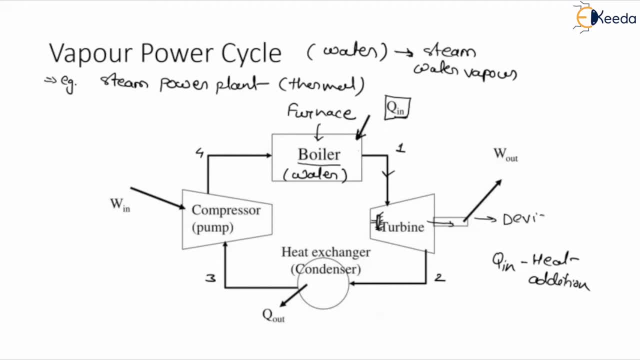 particular shaft is connected to another device like generator. So what will happen here? The high pressure, high temperature steam will hit the blades of the rotor. Rotor will rotate, It is connected to the shaft and that shaft will get the power from the rotation of rotor and that power 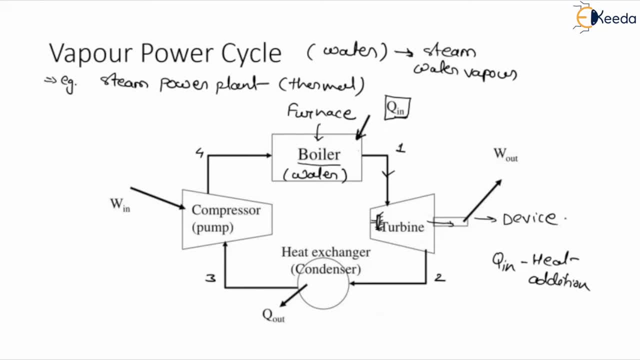 will be transferred to another device for another purpose. So what is happening here? We are giving work to another device. So what is happening here? Work output. we are getting What we are getting here: Work output. So with the help of turbine, we will get some work output. So this: 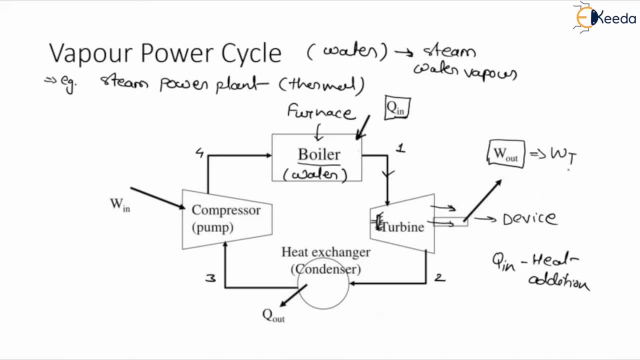 particular work or work output is called turbine work. So here what is happening? The boiler is going to transfer the high pressure, high temperature steam to the turbine and that steam is going to expand in the turbine. What will happen here? because of the shape of the turbine, It will expand and 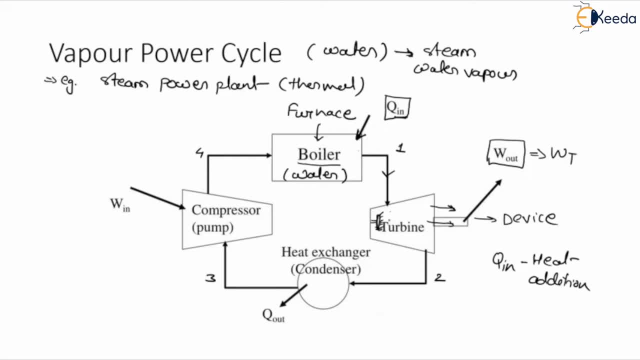 this expansion of heat we will consider in the turbine and it will produce some work that is called the turbine work or we can say as the shaft work. So here we are getting the work output from the turbine. Now, after this particular part, the remaining heat which is unused it will transfer to the condenser. So this is our process. 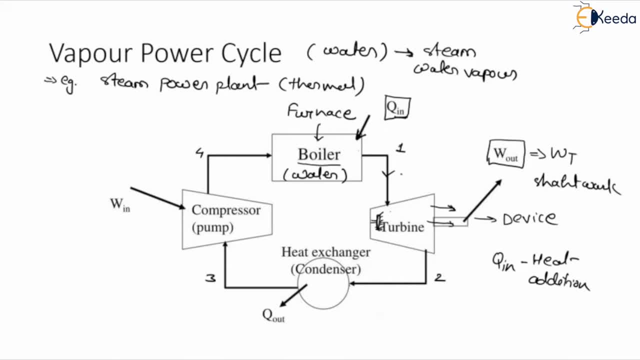 number 2.. So 1 to 2 we are considering, as the heat addition is happening in the boiler, Then it is transferred to the turbine and the remaining heat which is unused heat in the turbine, it will transfer to the condenser. So from 1 to 2 we are considering expansion of the steam only. Now the 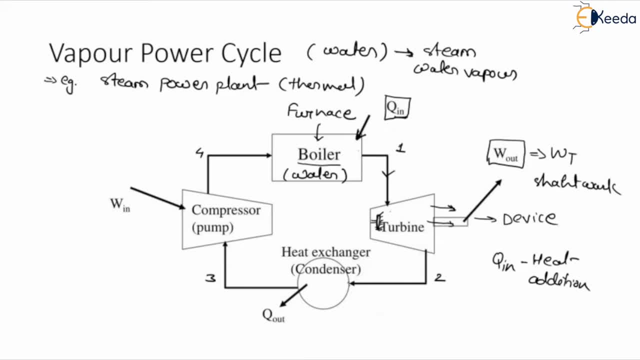 nous. And here we are consideringْ The cooler, the lower temperature steam will increase, so that the steam will be less as we will get the lower pressure, lower temperature steam in water vapor, But the steam that iság. So the steam leaves the turbine from the remaining steam and it will convert to the condenser. Steam isığて. So here the steam leaves the turbine from theanan, it will transfer to the isì, And here the steam kan Can, can conzervere into water vapor. the and the steam will drive here And it will transfer to the condenser, where steam condensed, and here the temperature and pressure will be lower compared to water vapor in the Tucson to low pressure will be lower, or compared to other devices. So here is the lower. maintained steam will have more heat, whereas the soil is not higher, So here we will get the lower因为지. 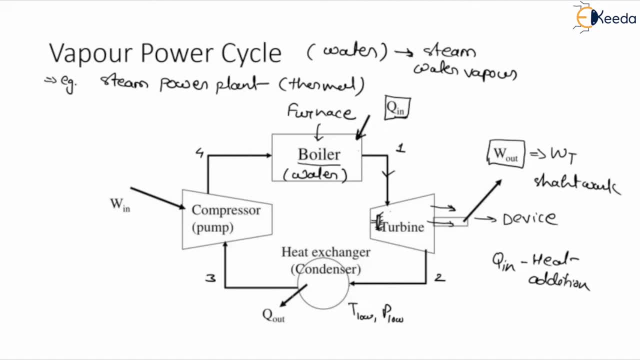 and it will condense into water and it will reject heat. So the heat output we are getting in the process of condenser. So this Q out is what It is: the heat output or heat rejection. So heat rejection we are considering in the condenser and the steam which is at the low. 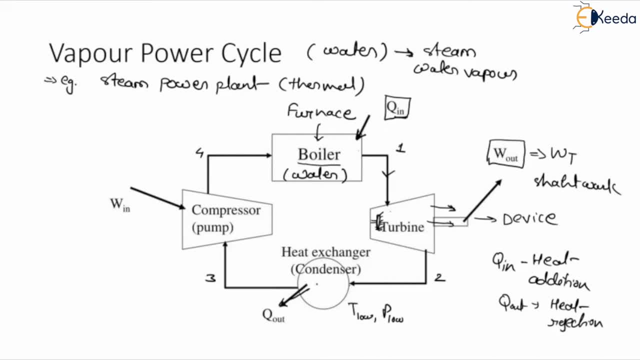 temperature, low pressure, will convert into the water, and when we get the water here in the condenser, So this water will pump back to the boiler with the help of compressor. So here we are compressing the water. So here we have to do some work over this particular part. So 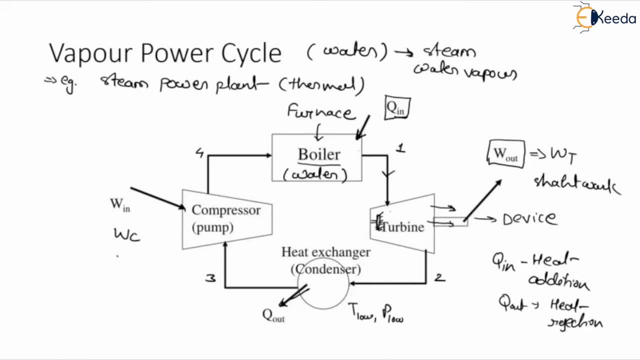 this is represented as compressor work or work input. This is defined as what Work input. So we have to do some work over this device to pump the water from condenser to the boiler Now. this remaining water will use here in boiler to convert into the steam Now. 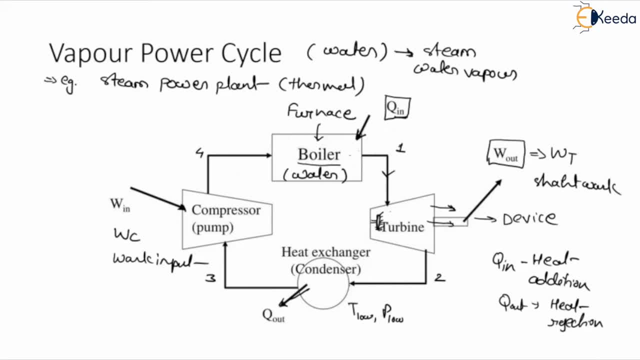 that steam we will transfer again to the turbine and this turbine will expand the steam. It will produce the shaft work. Then remaining heat will again transfer to the condenser and then it will convert into the water. Then it will goes back to the boiler with the help of. 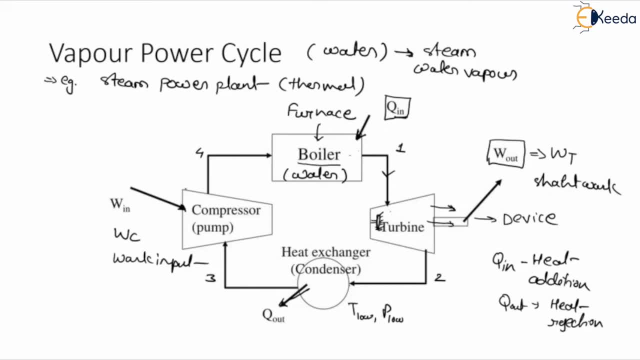 compressor or the pump. So this is the cyclic process. This process will continue. So this is what This is a type of cyclic process. Here the water will continuously convert into steam: It will expand, Then it will condense, Then it will compress and then it will use. 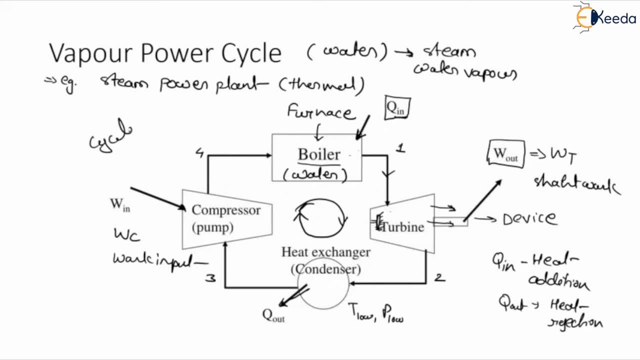 continuously. So this is what This is: a cyclic process. So in cyclic process, if the fluid is undergoing- or we can say the fluid is undergoing- a cyclic process, in that condition there will be no net change in internal energy over the cycle and here the net heat. 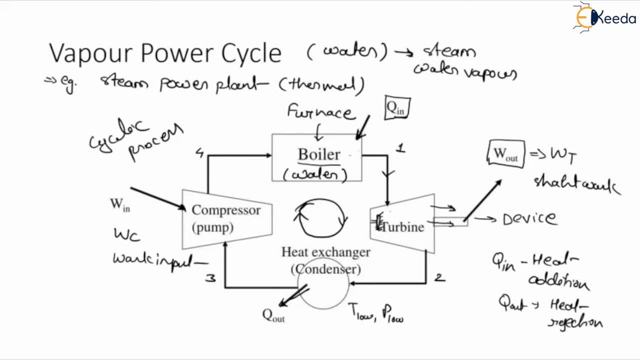 transfer as the heat during the cycle. it will be equal to net energy transfer as work, and this work we are getting from fluid. So what is happening Here? there is no internal energy. we are considering No net change in internal energy, Only net heat. 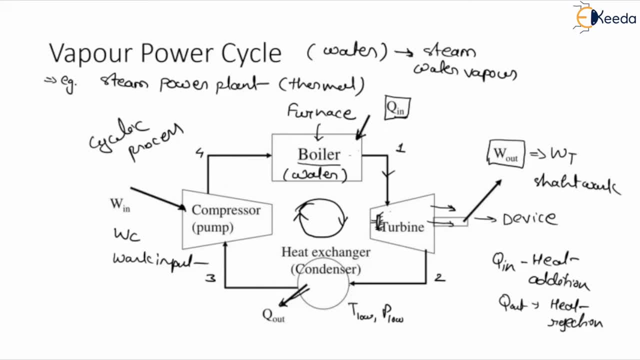 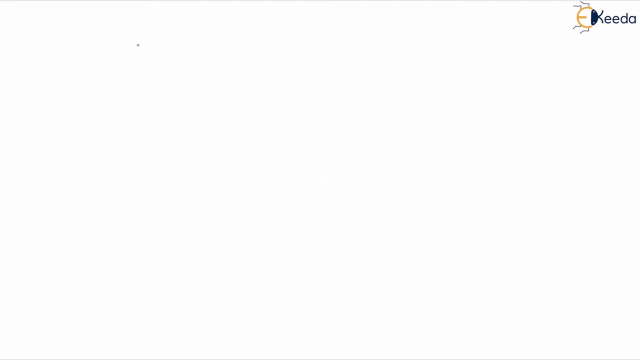 energy transfer as heat, it will converting into work which is getting from the fluid. So net heat transfer as heat will be equal to net energy transfer as work. So in the cyclic process we can write as Q for the cyclic process it will be equal to W net for the cycle. So summation of Q or this is also defined as Q net. 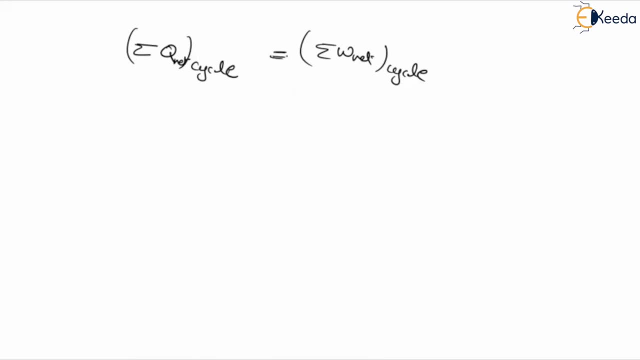 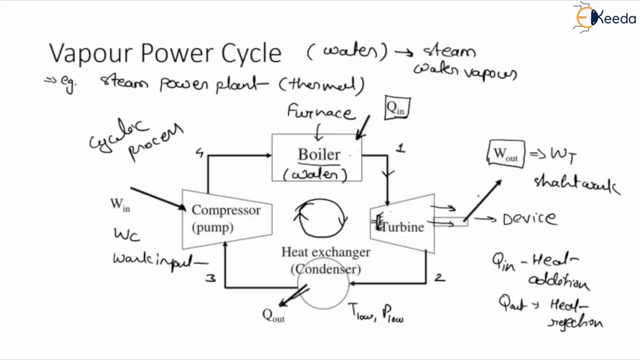 So summation of Q net for the cyclic process will be equivalent to summation of W net for the cyclic process, where this W net we can define as the difference of turbine work and the pump work. So this is our turbine work And here this compressor work, or we can define as pump work. 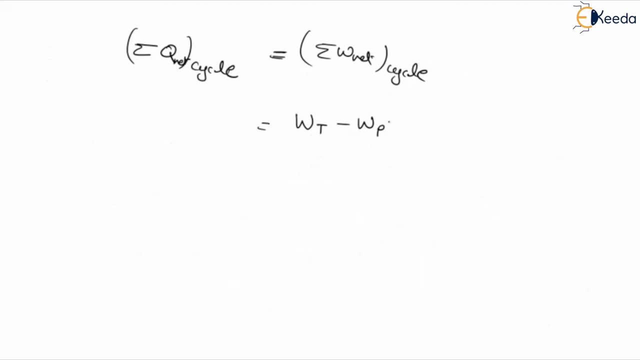 So net work done will be what Wt minus Wp, which is the net work done we are getting from the steam power plant. So here this Q net we can define as Q1 minus Q2. that will be equal to Wt minus Wp. 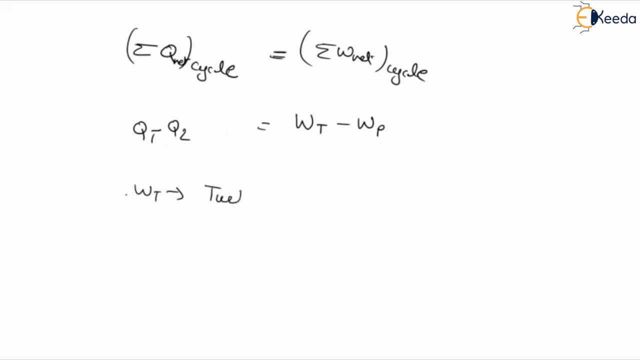 So here Wt is what It is the turbine work, Or work transfer from working fluid, And Wc or Wp is pump work, Work transfer to the working fluid. So this is all about for the cyclic process, And here Q1 and Q2 is what 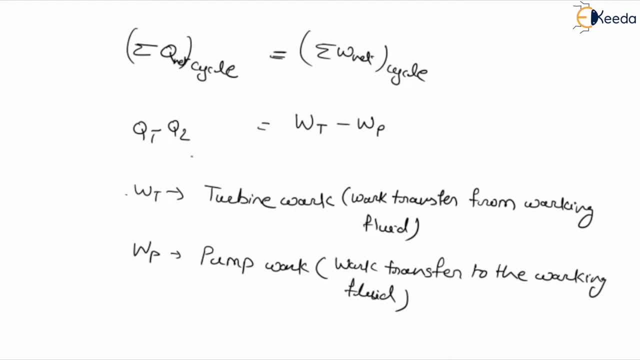 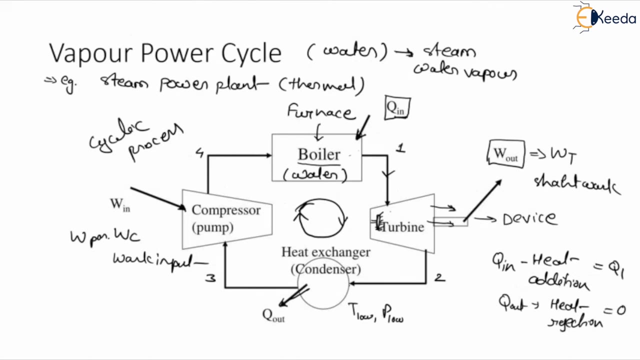 Q1 is the heat transfer to the working fluid And Q2 is the heat rejected to the working fluid or heat rejected by the working fluid. So basically, Q1 is what Heat addition I have written here. So Q in we will consider as the Q1 and Q out we will consider as Q2.. 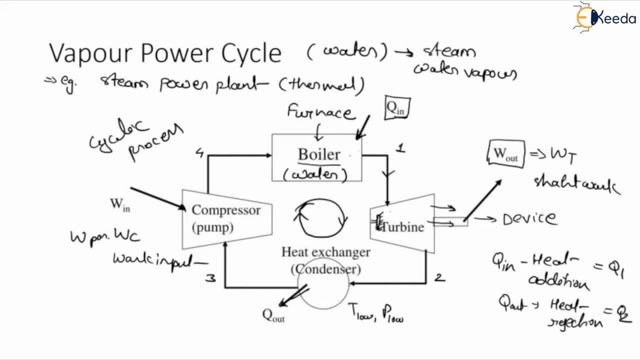 So these terms we can define for the cyclic process where the water is converting into the steam And then steam is producing some work, As the shaft work, and the heat is directly converting into work. So this is about the vapor power cycle where the working fluid is vapor or water. 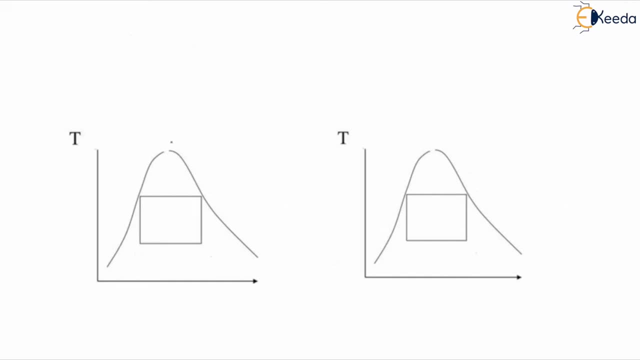 Suppose, if we want to represent the working of the steam power plant on TS diagram. So suppose here we have TS diagram, TS diagram, TS diagram is what Temperature entropy plot. So temperature entropy plot we will define on the basis of working of the steam power plant. 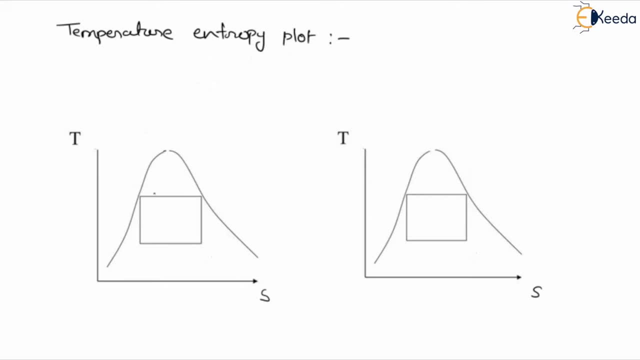 So suppose here you can see, this is the dome, This dome. This dome is representing what This dome is representing: the phase change of working fluid. So here this is representing what This is a dome And this dome is usually represent the phase change of the working fluid. 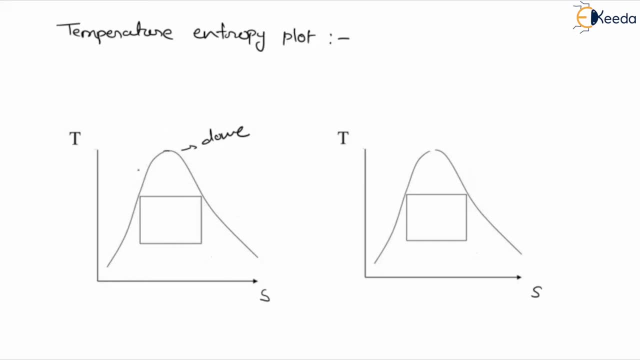 So every phase of the working fluid, that is, the water, we will define on the basis of this curve of the dome. So here, in this particular dome, inside this dome, we will consider a region which is the combination of liquid and vapor. This we have learned in the phase change of the. 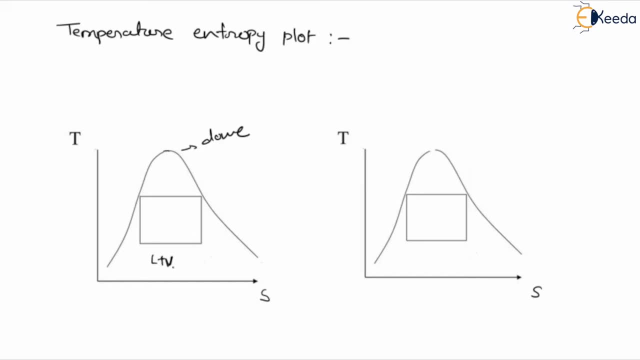 Pure substance. So inside the dome it will be liquid plus vapor region. Now, right side of it It will be completely vapor or purely superheated steam. So here in this right side, the steam will be in the vapor form or it will be purely superheated steam. 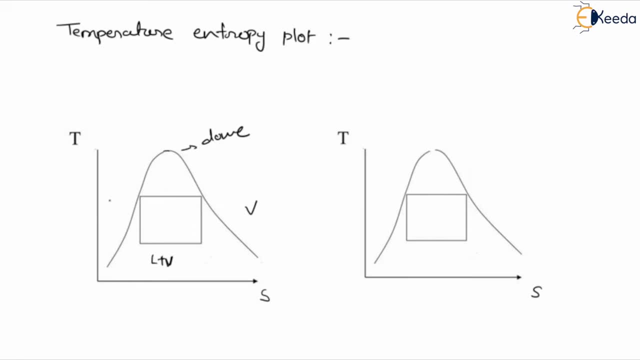 And at the left side we will consider compressed liquid. So this is the liquid region, This is liquid plus vapor region, And this is vapor region. Now this line, This particular line over the dome, is represented as saturated liquid line, where the liquid will start converting into the vapor. 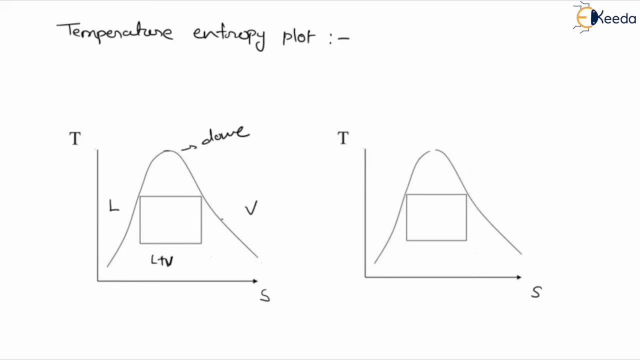 And here this line is known as the saturated vapor line, where the vapor will completely form and it will start superheating from here Because the temperature is going beyond the 100 degree centigrade. So this is the liquid plus vapor region: 100 degree centigrade. 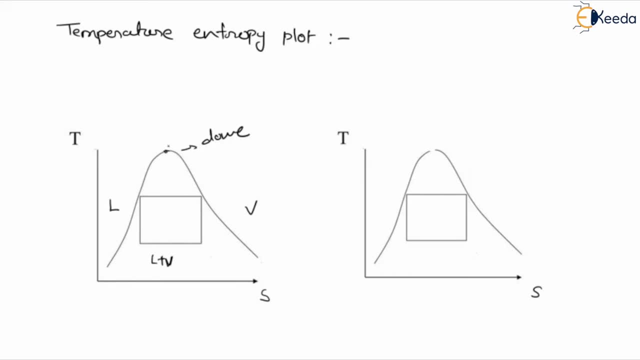 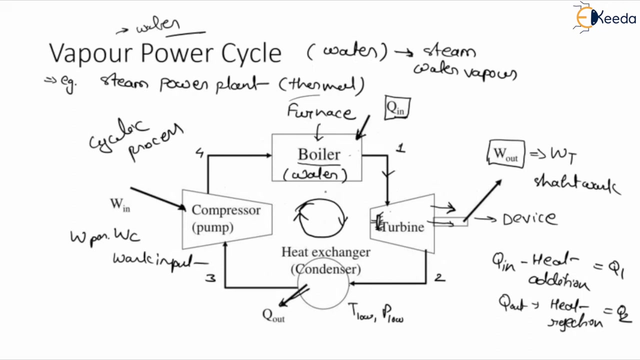 And where these two lines will meet. that is called the critical point, where temperature will be maximum. So this is about the pure substance diagram of phase change of the pure substance or any kind of working fluid. So, as per this diagram, In this boiler we are producing high pressure, high temperature steam. 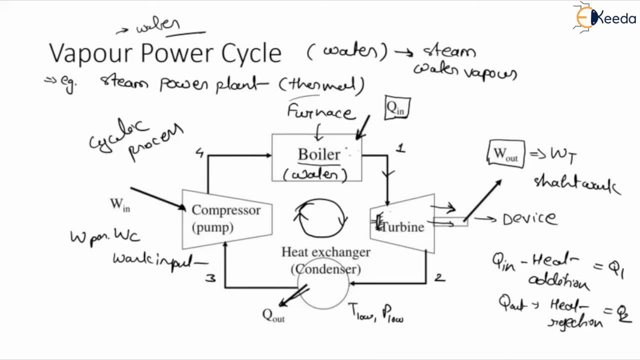 And this high pressure, high temperature steam Is transferred to the turbine And the turbine will expand the steam And it will transfer The remaining heat, will transfer to the condenser. So at condenser we are considering low pressure and low temperature steam. 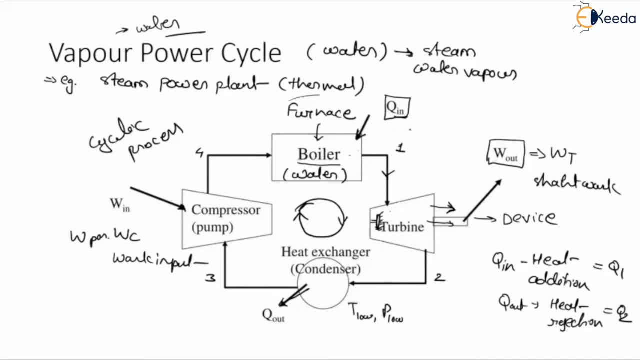 So boiler will be at high pressure, high temperature And the condenser will be at the low pressure and low temperature region. So in steam power plant This is a cyclic process. So steam power plant basically operate in a closed cycle Because here some working fluid which is used throughout the cycle or the process. 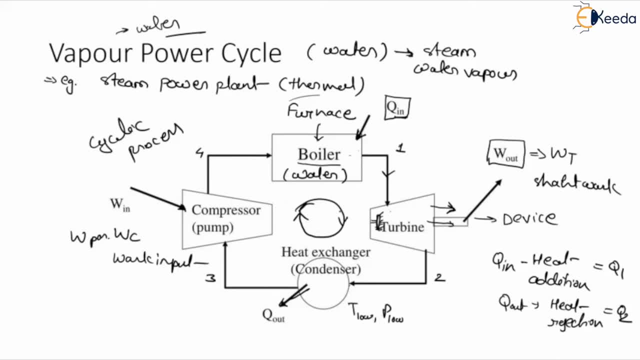 So the chemical composition of the working fluid does not change in this particular region. It will remain same. So this is a cyclic process And here this particular process we are considering as a closed cycle Because of the working fluid. If we are considering open cycle, 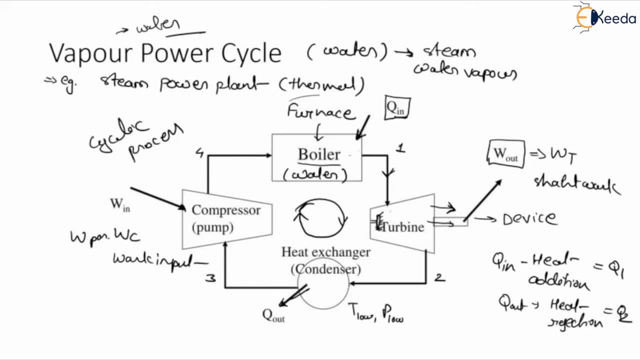 So here working fluid will not be in the liquid form Or it will not be in the vapor form Here because of the working fluid. We are considering this complete cycle as a closed cycle, And chemical composition should not change. Chemical composition should be same here. 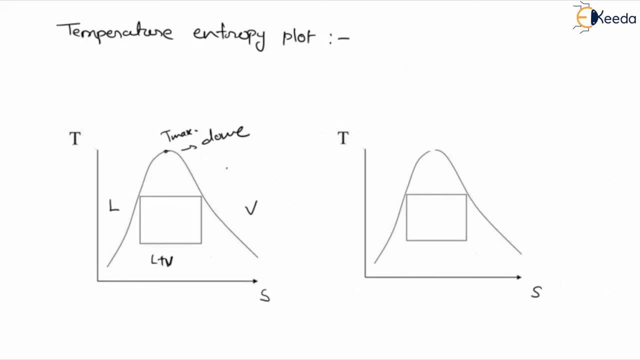 Now coming back to the temperature entropy plot. So I have told you about the phase change of the working fluid. Now, in this particular curve You can see. This curve is representing the pressure in the boiler And this is constant pressure curve. Here you can see this particular line. 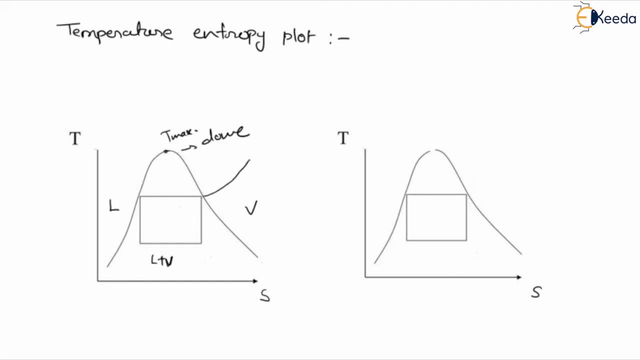 So if we form a curve here In the form of various properties, So let me extend this line So you will understand better. So suppose we have pressure here at this point, Because this is a T-S diagram, temperature entropy plot, So we can define only the values of temperature and entropy only. 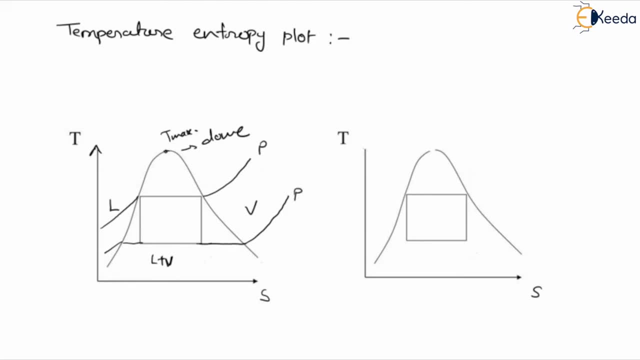 So suppose here, if we want to define the pressure, So here you can see, This is the curve, This is our dome, basically, And here we are going to define the curve on the basis of different properties. So here you can see this particular curve. 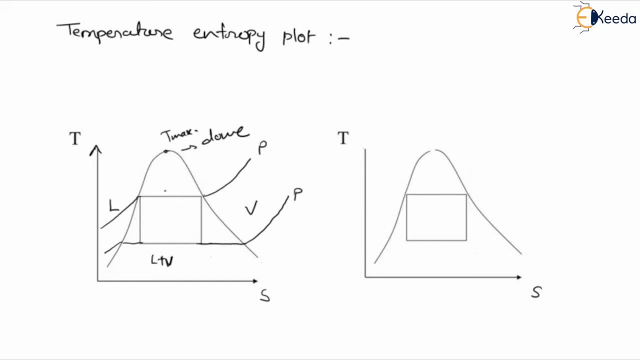 Or this line, Or this curve, Anything you can take. So this line is representing what It is representing: constant temperature. But here you cannot see the pressure will be variable or not. So in this particular condition, if we want to define the pressure, 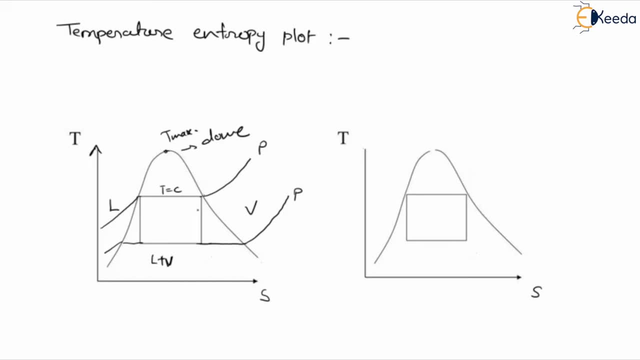 So pressure in the boiler It will be at constant condition. The pressure will be at higher side But there will be constant pressure. So this particular curve will be defined as the constant pressure curve. But in this condition you can see After this particular point. 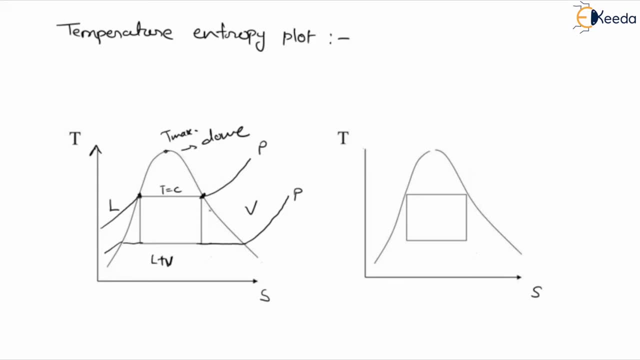 Between this and this, the temperature is constant. But at this particular point, If you see the curve, So it is representing the increase in temperature. So the temperature is variable here. So here, in this particular condition, the pressure will be constant throughout. But from here to here the temperature will be constant. 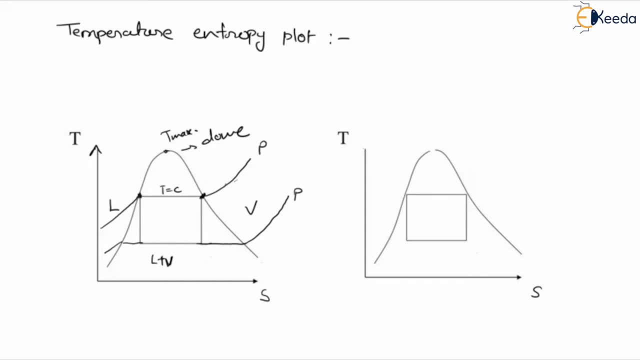 And from this point, after this point, the temperature will be variable. So this particular curve is representing the variable temperature with constant pressure. Now the second curve is representing the pressure in the condenser. So here, from this point to this point, The pressure will be constant, or from this point to this point, the pressure will be constant. 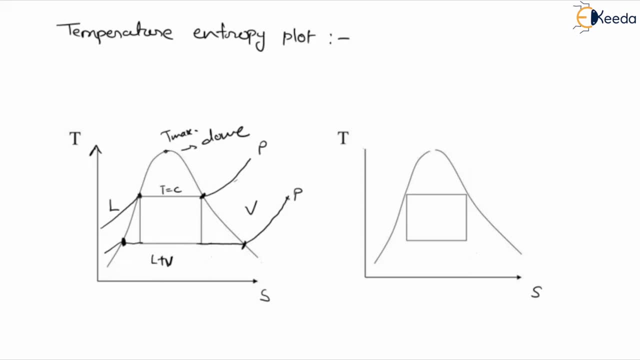 But temperature will increase from this point or beyond this particular point. Why? Because it is the superheated condition. It is what It is the superheated condition. So here the pressure is constant and temperature is changing continuously. Now, if we extend this constant temperature line, 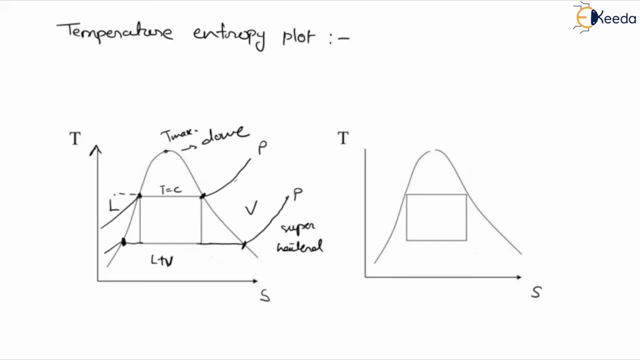 From this point to this point. So it is intersecting this vertical temperature line. What is happening here? If we are extending this line, then it will intersect this vertical line. So this point is represented as the boiling temperature Tb. What is this? 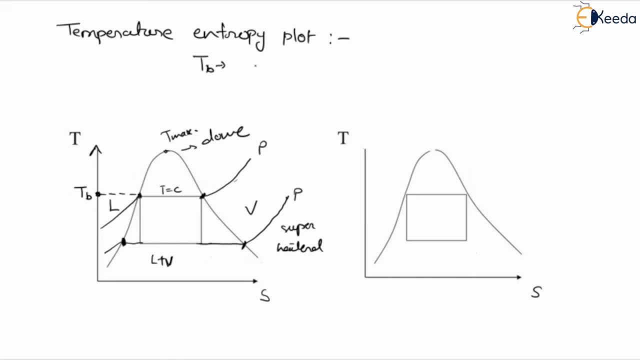 Tb. So Tb is what, Tb is the boiling point, Boiling point of water. At this particular point the water will boil. So boiling point of water And this boiling point of water we will define on the basis of pressure of boiler. 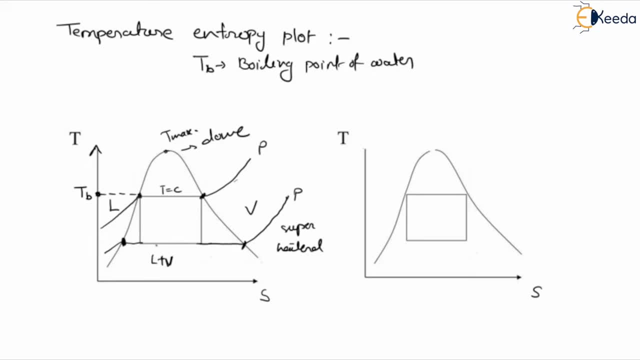 Corresponding to pressure of boiler. Now, similarly here in condenser, if we extend this line further Towards left, So we will define one temperature here. So it is defined as the Tc Condenser temperature. It is known as the saturated temperature. 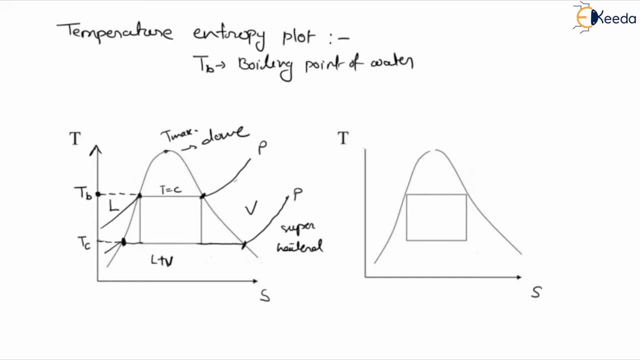 So the Tc is known as what Condenser temperature or saturated temperature, And it will be corresponding to pressure of the condenser. Here this will be corresponding to pressure of boiler And this will be corresponding to pressure of temperature. So here what is happening. 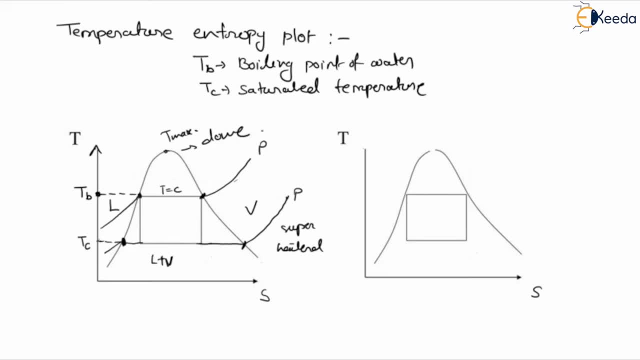 Heat is added by the boiler. So in this particular condition we will consider heat addition through boiler, that is QV, And in this condition the heat rejection, So it will be Qc as the heat rejected by the condenser. So this is about the temperature pressure diagram. 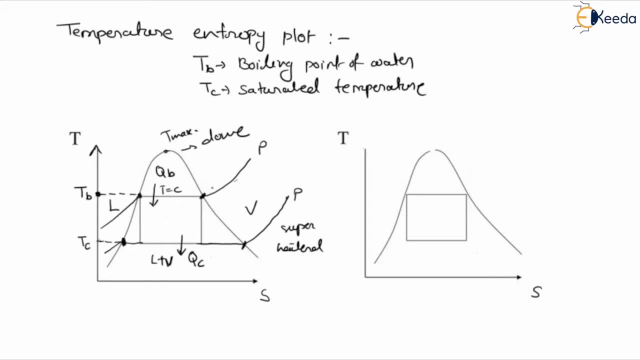 Or the variation of pressure and temperature. Now, if we define the complete cycle of the steam power plant, So it will be defined on the basis of 4 processes only, And here this complete cycle is known as the theoretical cycle, Which is representing the each and every phase of the steam power plant. 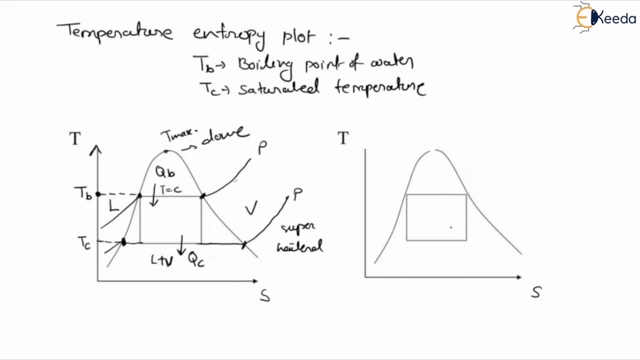 So here, if we write down all the phases of the steam power plant, So it will be defined as: So this is our point 1.. This is our point 2.. This is our point 3. And this is our point 4.. 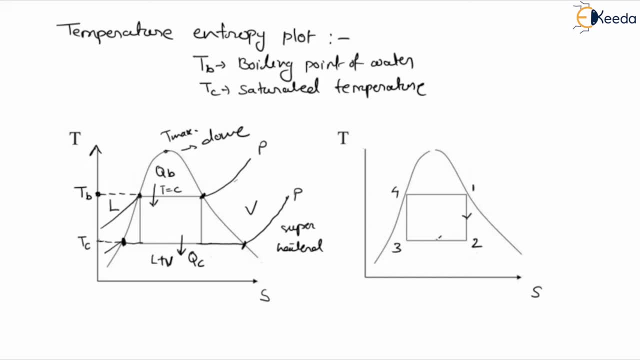 So in this particular condition we can say: And the process is the cyclic process. So here the cyclic process we can define on the basis of arrow. So this 1 and 2 is representing what It is, representing the expansion process. So it is called the isentropic expansion. 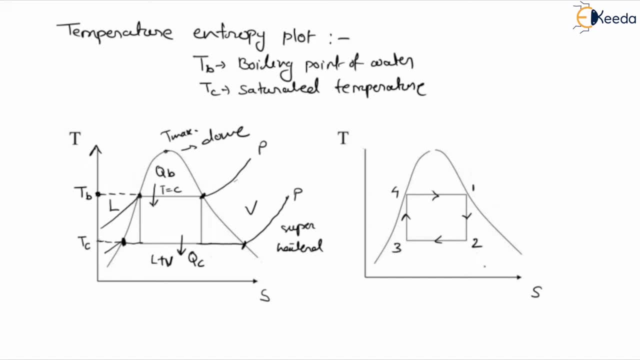 Why? Because the entropy is constant here. This is the T-s diagram. So this constant 1 to 4 is representing what Constant temperature. Constant temperature we always defined as the heat addition. So heat will be added here in the form of Q. 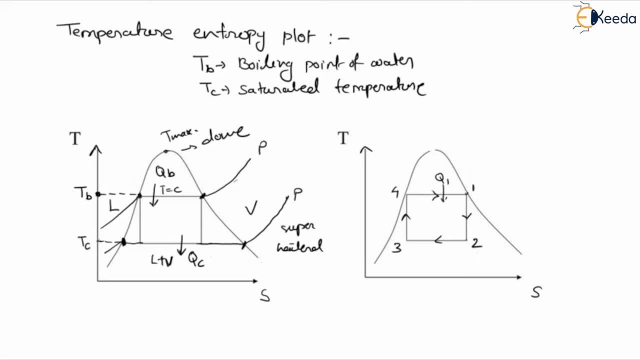 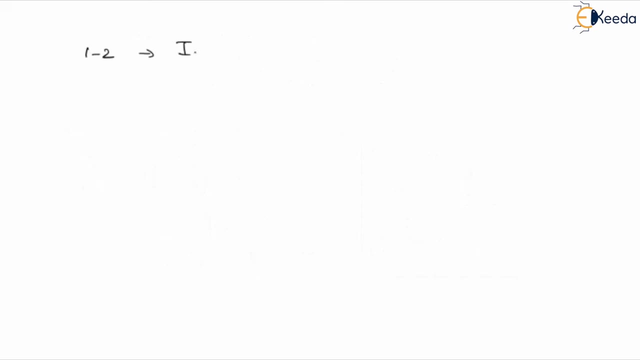 Now, from point 1 to 2 we are considering the turbine process. So from 1 to 2 the steam will expand, And the steam will expand isentropically. So here we can write down this term as 1 to 2, as isentropic expansion. 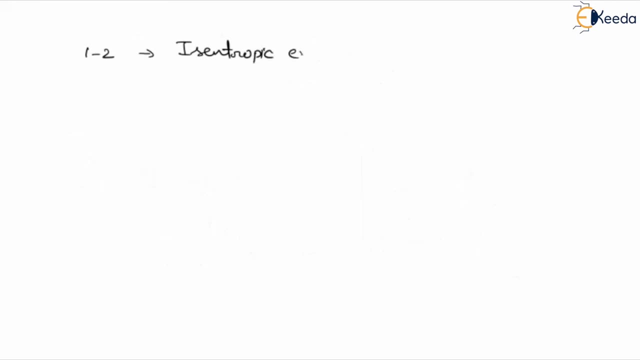 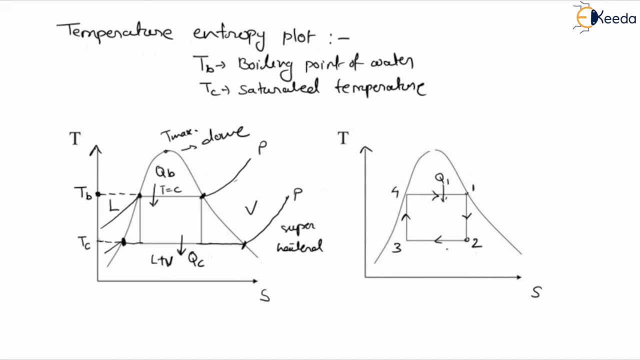 It is called isentropic expansion. Now, from 2 to 3. what is happening? The 2 to 3 heat rejection is happening through the condenser, So it is called constant temperature heat rejection. So heat will be rejected in the form of Q2.. 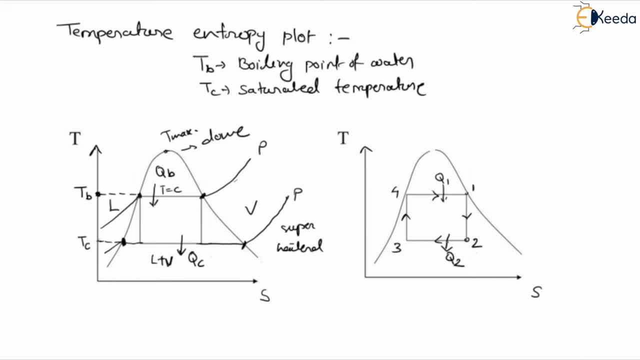 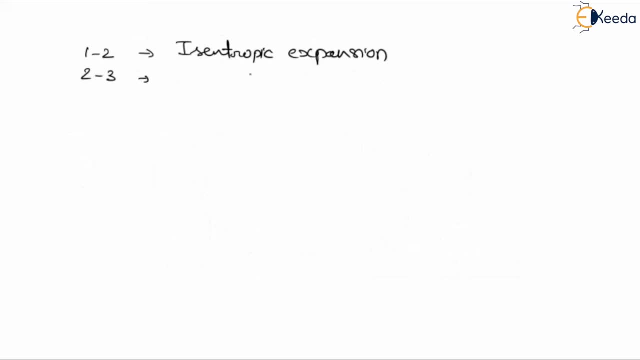 And it will happen on constant temperature. So 2 to 3 is defined as what? Constant temperature, Constant temperature heat rejection Or constant temperature heat rejection. we can say isothermal heat rejection also. Now, from 3 to 4, we are considering compression of steam. 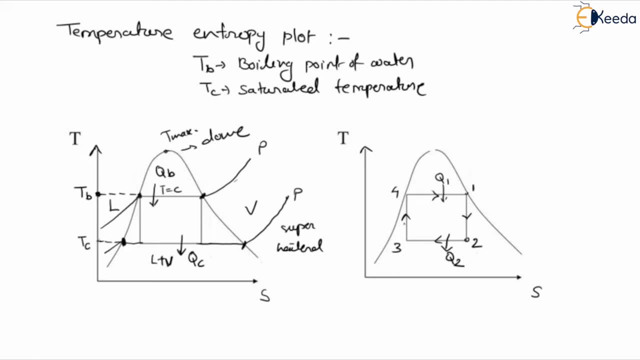 So this compression of not complete steam- It can be the combination of water and water vapor Or it will completely convert into the water because of the condenser. So 3 to 4 we are considering as the isentropic compression to pump the water to the boiler. 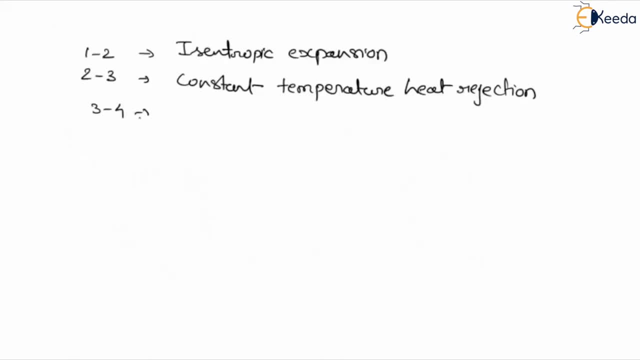 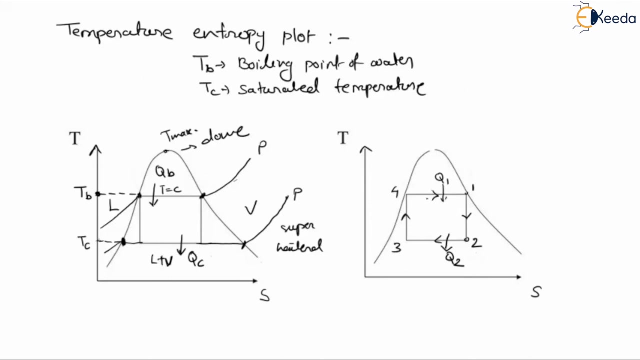 So 3 to 4 is defined as isentropic compression And here the entropy will be constant. Temperature will be variable, but entropy will be constant. Now here, from 4 to 1, what will happen? Constant temperature, heat rejection into the boiler. 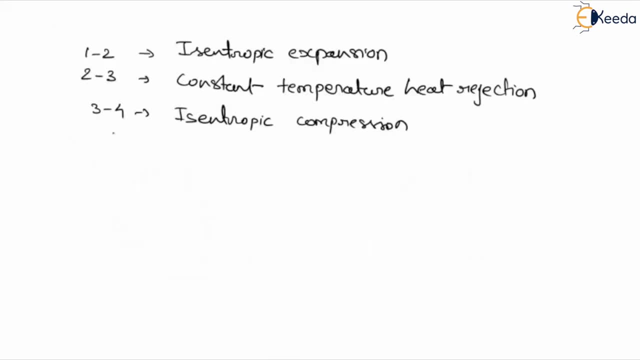 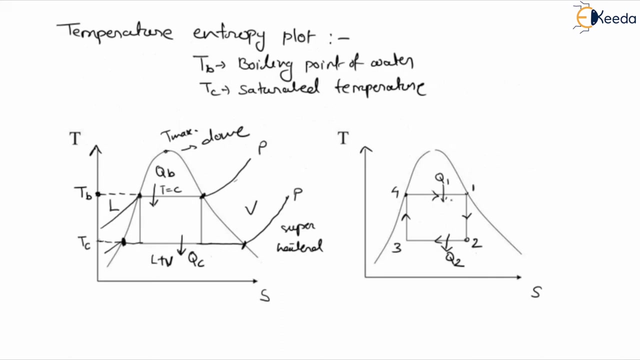 So this 4 to 1 we are considering as constant temperature heat rejection. So it will be what It is also called isothermal heat rejection. So this is what This particular cycle is, the theoretical thermodynamic cycle, And this cycle is independent of working fluid. if we say, 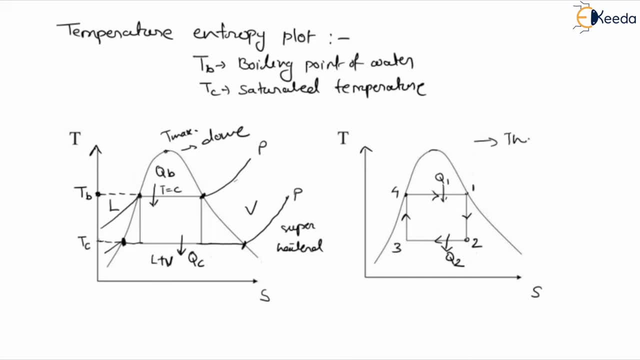 So this particular cycle we can define as theoretical cycle And this theoretical cycle is usually independent of working fluid. So theoretical cycle we can compare with the ideal cycle also, But ideal cycle we usually defined as the Carnot cycle. Ideal cycle is what? 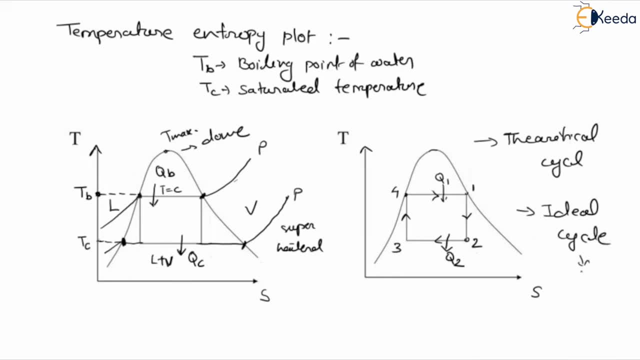 Where we are getting 100% efficiency. So this particular cycle will be defined as Carnot cycle. But there is no engine can operate between two heat reservoir can be more efficient than a Carnot engine operating between the same heat reservoir. So if we are using practical data, so we will get the actual cycle only. 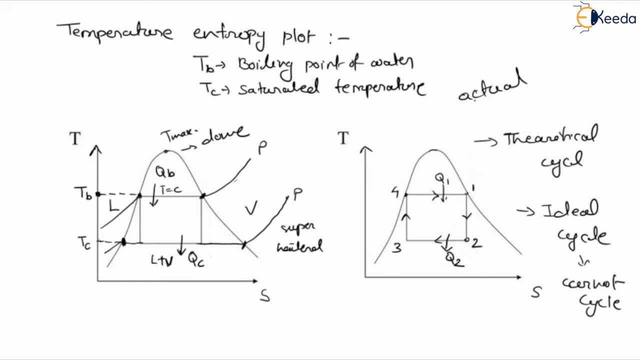 But if we are considering the ideal data, So we will get the ideal cycle that is called as the Carnot cycle. So this is what this cycle is represented as: thermodynamic theoretical cycle, which is independent of the working fluid, And this is the most efficient cycle for converting the thermal energy into work. 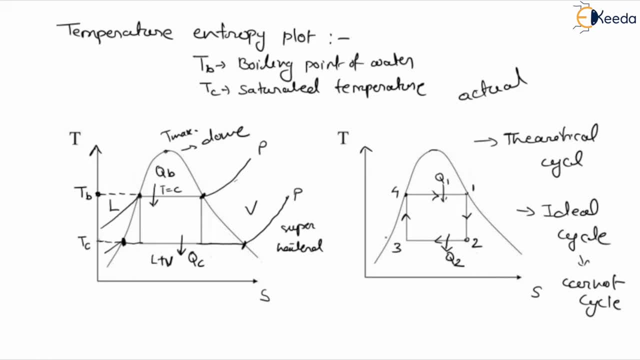 But Carnot cycle cannot be achieved in reality Because it's an ideal cycle. But the efficiency of the actual cycle we can improve by attempting the Carnot cycle more closely. So this is what this particular cycle we are considering as the ideal cycle, which is working over the substance. 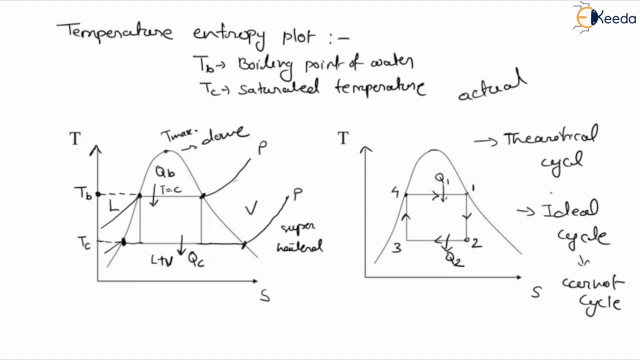 Here we are considering a working substance which is getting heat. It is transferring the heat to a particular device and that is producing a work, or it is giving some work output. So here we are considering a working substance. So here we are considering the heat transfer to a particular device and that device is converting heat into work. 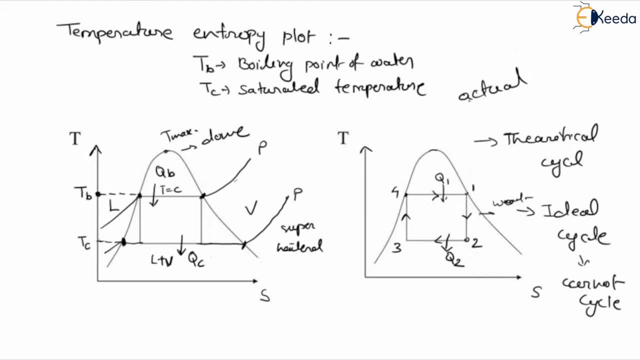 And this is a cyclic process, so it will be continuous. So here, if we want to talk about the steam power plant, So steam power plant can also operate on the Carnot cycle closely, But not as it is. So we can improve, We can do some improvement in a particular type of steam power plant. 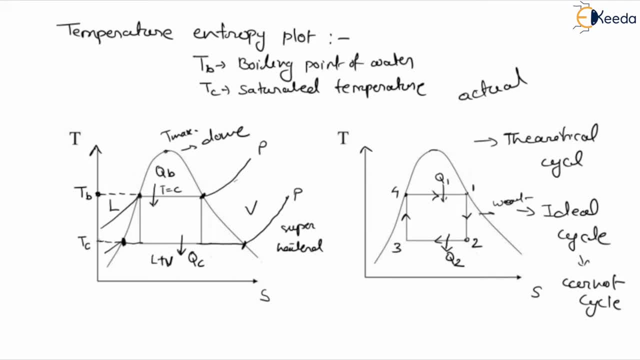 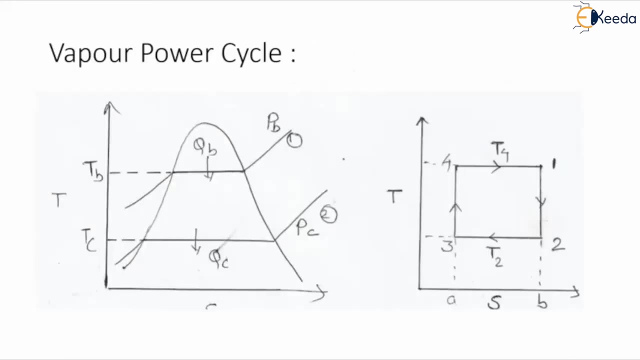 To get the efficiency like Carnot cycle. But we cannot get 100% efficiency as Carnot cycle. We can try to get more efficiency by some improvement or by some changes. So here you can see this particular cycle Now. here you can see a process of the steam power plant. 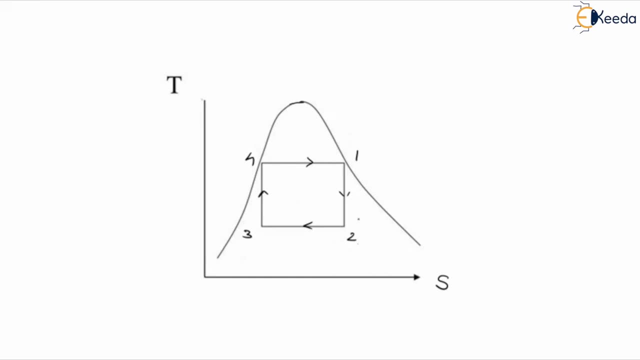 Where 1 to 2 is what It is, the isentropic expansion, 2 to 3 is constant temperature, heat rejection, 3 to 4 is compression isentropic And 4 to 1 is the heat addition at constant temperature. 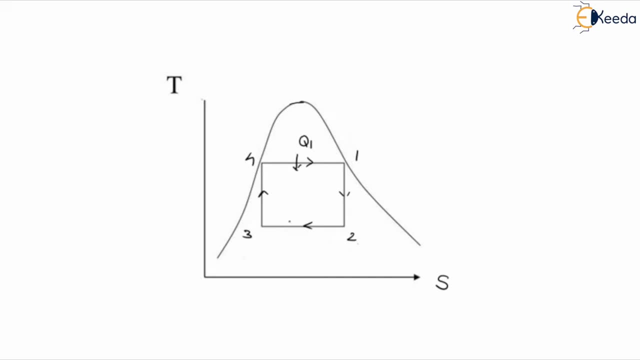 So 4 to 1 we are considering heat addition, 2 to 3 is the heat rejection, 1 to 2 is the turbine work And 3 to 4 is the pump work or compressor work. So here let me write down the processes. 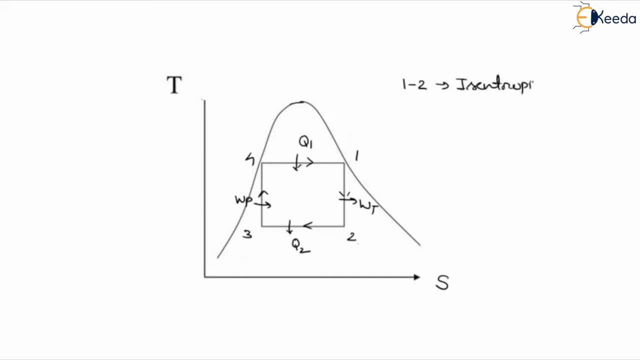 1 to 2 is isentropic expansion, 2 to 3 is constant temperature heat rejection, 3 to 4 is isentropic compression And 4 to 1 is constant temperature heat addition. So here you can see. 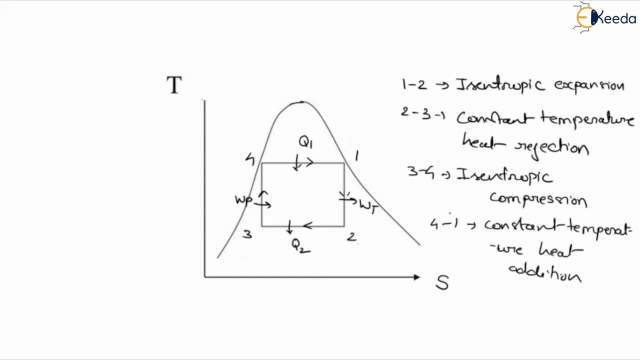 So there are 4 processes we are considering in the cycle of the steam power plant, And this is what This is the TS diagram. So basically here, entropy at 1 to 2.. Here you can see 1 to 2.. So entropy at this particular point will be same or it will be constant. 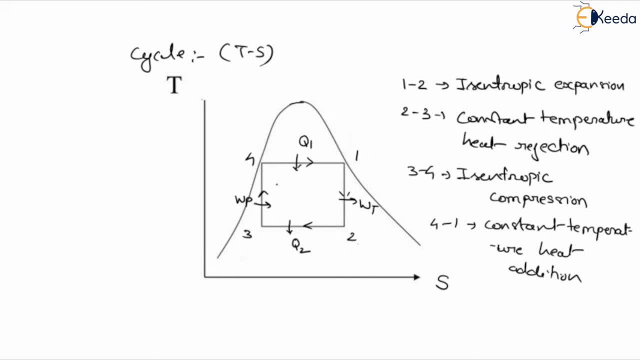 And 3 to 4, it will again constant, Because these 2 processes are what Isentropic processes. So here we can say: entropy at 1 and 2 will be equal, And 3 and 4 will be equal. So this is the ideal case. 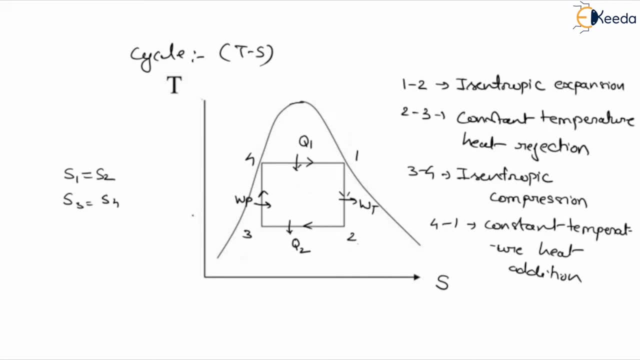 But practically the efficiency of the turbine and the pump is not 100%, So we will consider some losses here Because of this particular condition. We are considering this condition as the ideal condition, But practically this condition is not possible. So here we will define some losses. 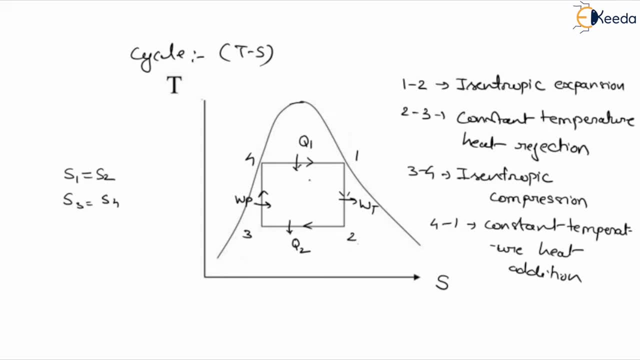 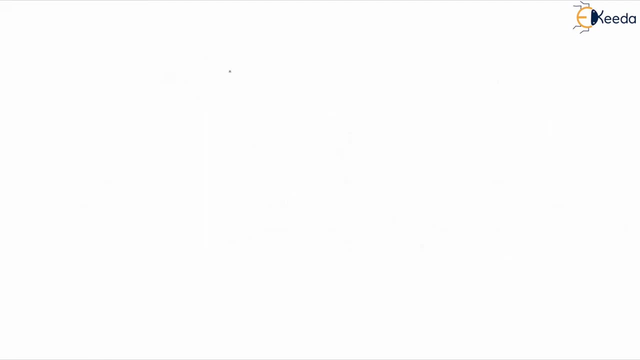 That will change the value of entropy. So here, if we define this particular process, Suppose if we are considering 1 to 2 dash, Suppose this is 1 to 2 dash And then 3 to 4 dash, So 1 to 2 dash. 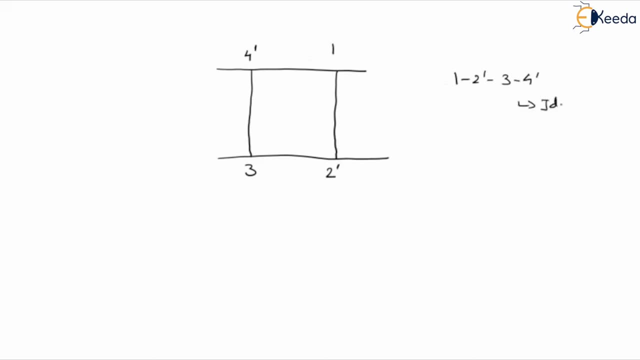 3, 4 dash, Suppose this is our ideal condition. This is what. This is our ideal condition. So here in this process, 1 to 2. This is isentropic compression, But in actual condition, If we are considering actual process. 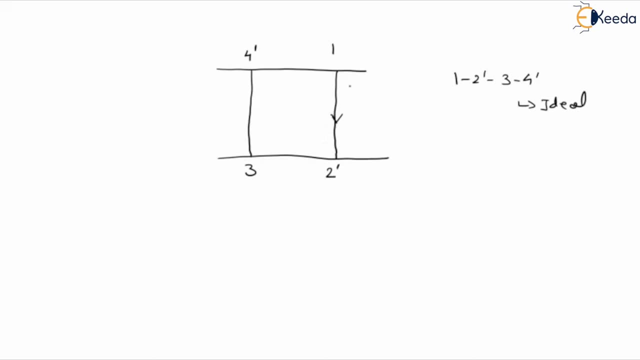 So this curve should not be a straight line. This curve will be like this, And this point I am marking as point 2.. So this particular 1 to 2 dash. So let me change the color So you will better understand. 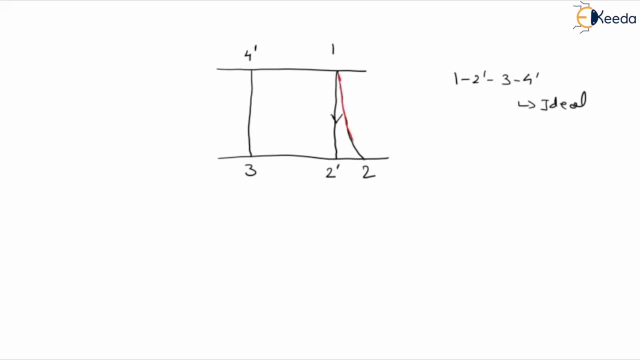 So this particular line- Suppose this red line- Is representing the actual process. So 1 to 2 dash is represented as isentropic compression Where the entropy is constant. But in this curve, If we are defining actual process, So this curve should not be straight. 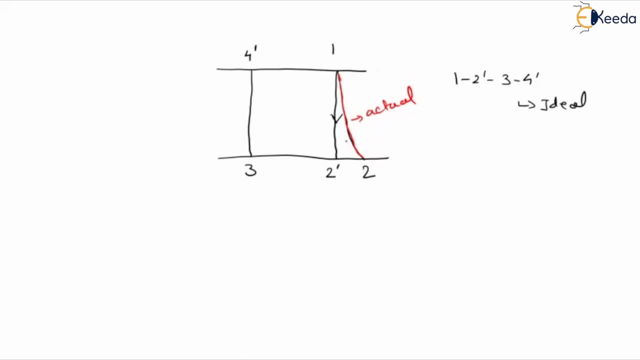 So 1 to 2 dash is representing the actual expansion. 1 to 2 dash is representing what Actual expansion? So in this expansion We are considering 2 processes: 1 to 2 dash and 1 to 2.. 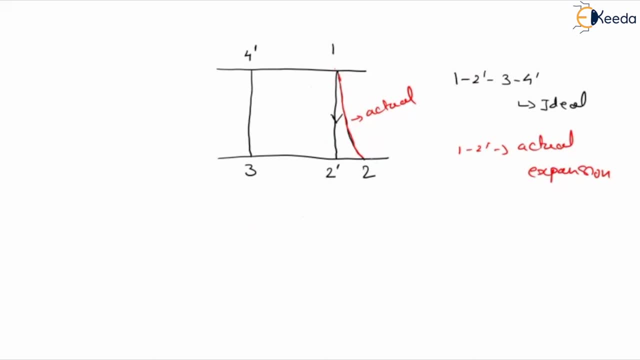 So in this condition, If we define entropy Or any kind of other properties, So suppose if we are defining entropy, So H2 will be greater than H2 dash, H2 will be greater than H2 dash. Similarly, if we define 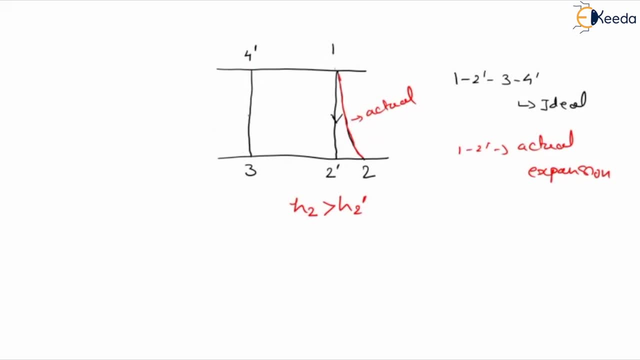 Entropies 3 to 4.. So 3 to 4 dash is defined as isentropic expansion. So in 3 to 4 dash. This is representing the ideal condition, But if we want to define the actual condition, So in actual condition. 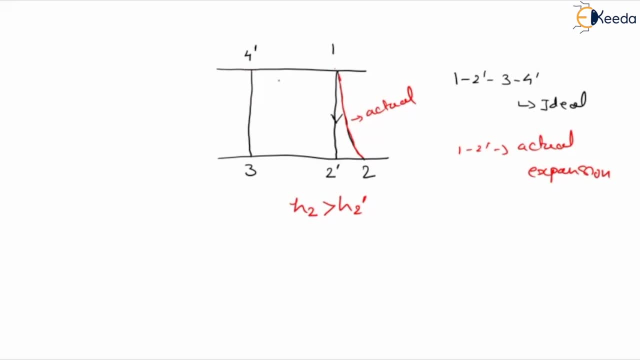 We have to define this. 3- 4 is not a straight line. It will be again a curve or some inclined line. So 3 to 4 we are defining as the expansion, Or the actual expansion Or actual compression. basically it will be. 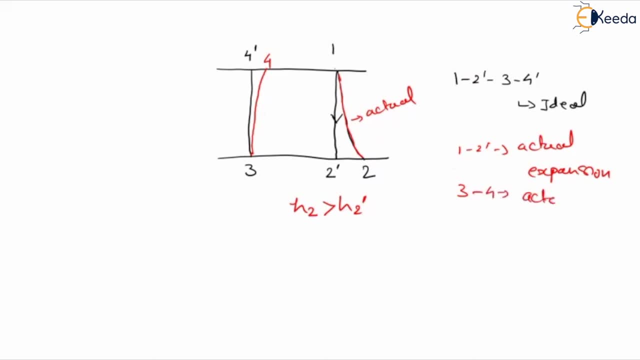 So 3 to 4 will be the actual compression. So actual expansion will be 1 to 2. And 3 to 4 will be the actual compression. So if we want to define In this particular condition, We can also say: 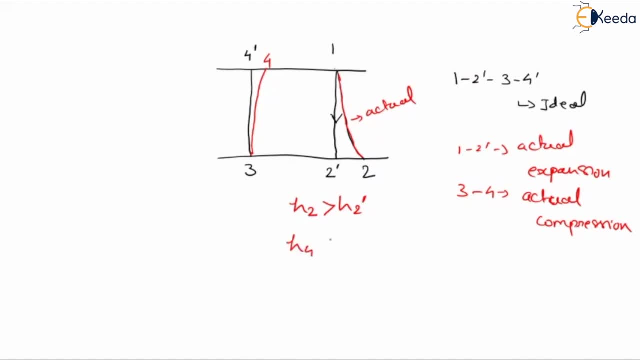 This H4 is lesser than H2.. 4 dash, Similar to this. Or if we define entropies, So S2 will be greater than S2 dash, Or S4 will be less than S4 dash. So if we want to define the work done, 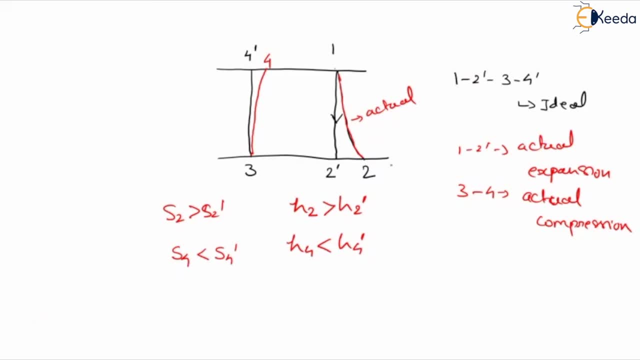 Work done during the process, So between 1 to 2. we are considering expansion work. So work done during process, 1 to 2.. Work done will be what? First we will define the work done: actual, So W actual or WT actual. 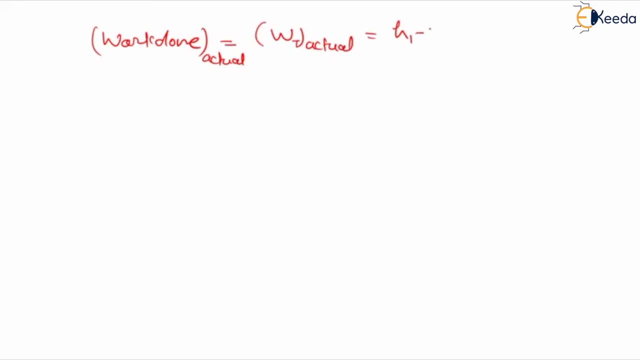 It will be equivalent to what H1 minus H2.. And if we are defining isentropic or ideal, Work done ideal Or isentropic. So let me write down WT ideal. So it will be defined as H1 minus H2 dash. 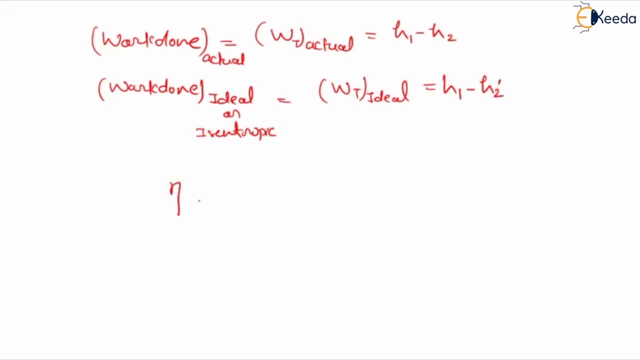 So if we define the efficiency, So efficiency will be what It will be defined as: actual work Divided by isentropic work. So it will be defined as H1 minus H2 divided by H1 minus H2, dash. 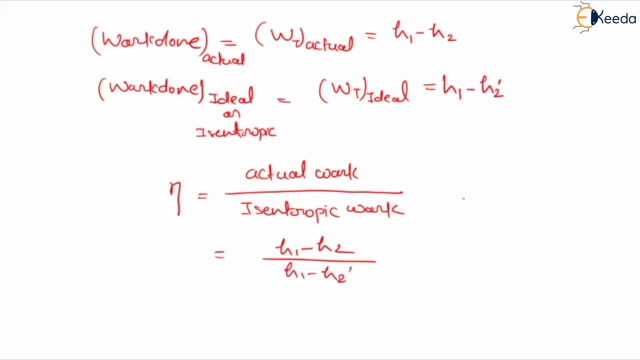 So where the isentropic work is greater than WT, isentropic or ideal, It should be greater than actual work. So this is what the process 1 and 2.. Similarly, if we define process 3,4 and 3,4, dash. 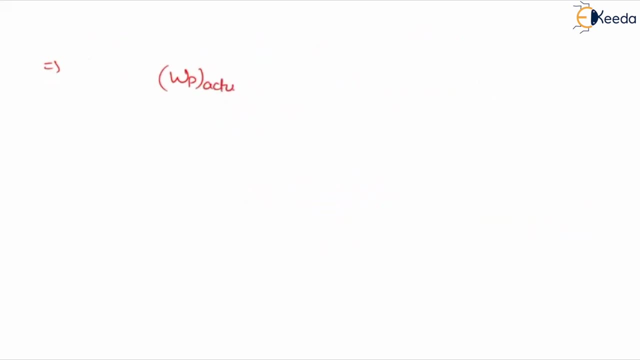 So WP pump work actual will be what Actual pump work will be defined as H4 minus H3. And the isentropic work we can define as what It is defined as H4 dash minus H3. So the efficiency here.